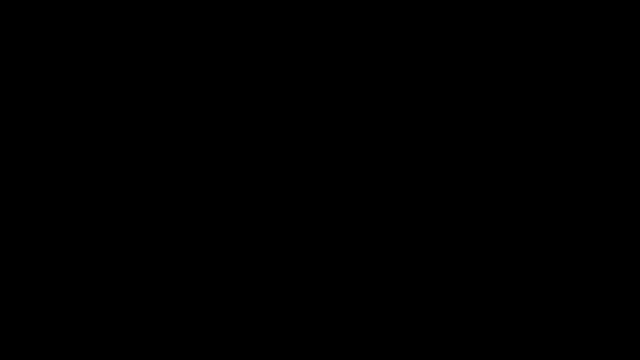 Now sometimes you need to write the quadratic equation given the roots or the solution to the quadratic equation. So let's say the solutions are 2 and negative 3. What is the quadratic equation in standard form? So first write it in factored form. If x equals 2, then the 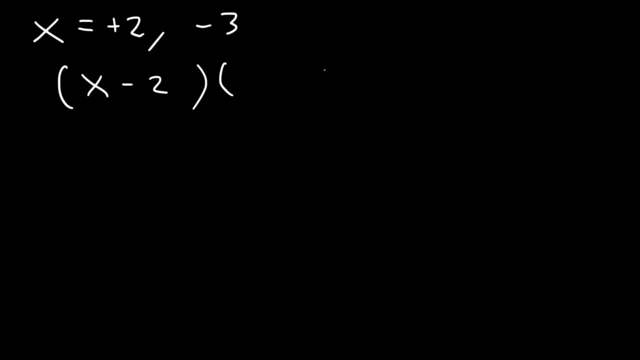 factor is x minus 2.. Change the sign. If x is equal to 3, then the factor is x plus 3.. After that you can just FOIL it: x times x is x squared, x times 3, that is positive 3x. And then negative 2 times x is negative 2x, And finally negative 2 times 3, that is. 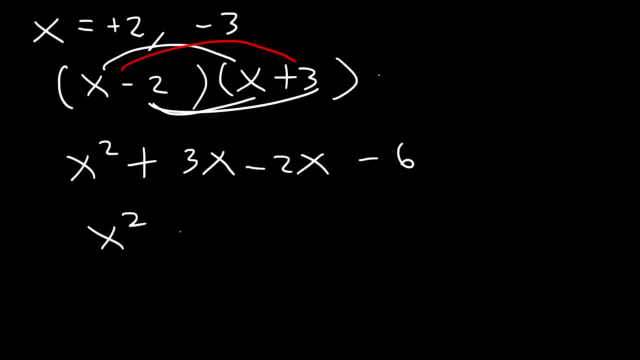 going to be negative 6.. Now 3x minus 2x is x. So this is the quadratic equation: x squared plus x minus 6. And we should have an equal to 0 somewhere. try this one, let's say: if x is equal to 3 and 2 over 3, 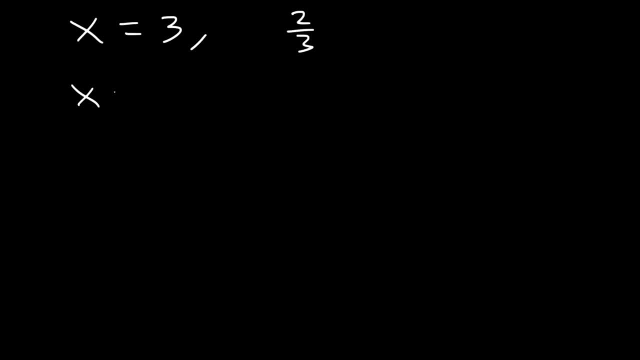 so what you could do is write both equations. for this one, let's subtract both sides by 3, so x minus 3 is equal to 0. that's one of the factors. for the other one, if we subtract both sides by 2 thirds, we'll have x minus 2 over 3 is equal to 0. now we want to get rid of the. 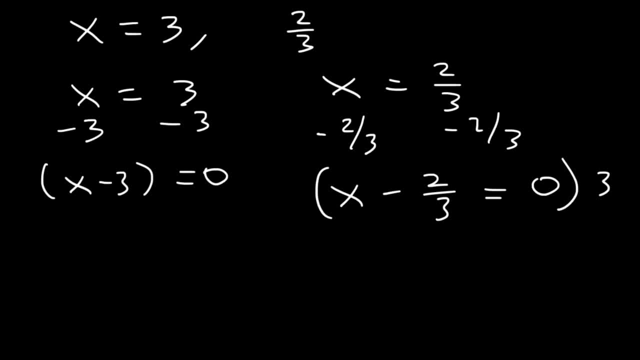 fraction. so let's multiply everything by 3, so 3 times x, that's 3x, and 3 times negative, 2 thirds, that's a negative 2. the 3s cancel 0 times 3 is 0. so here's the other factor. so in factored form, 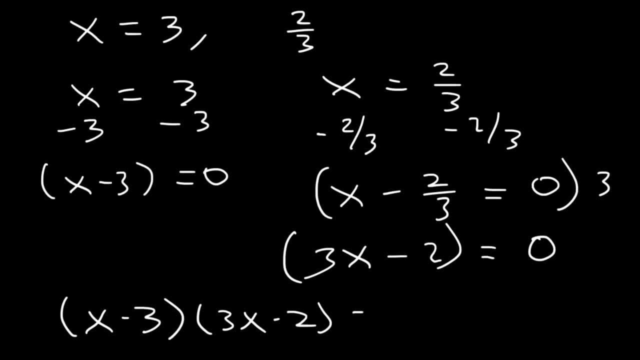 it's x minus 3 times 3x minus 2. so now we can go ahead and foil the equation for the other one. so we're going to write both sides by 2 and 2 over 3 expression. so x times 3x, that's 3x squared. x times negative 2, that's negative 2x, and then 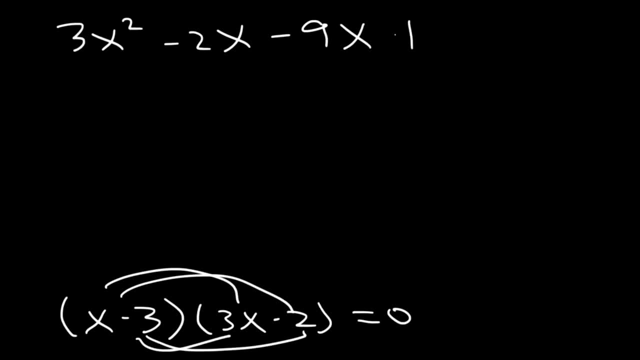 we have negative 9x and negative 3 times. negative 2 is plus 6. now negative 2 minus 9 is negative 11, and so this is the solution. now, what about this one? let's say, if you're given just one of the. 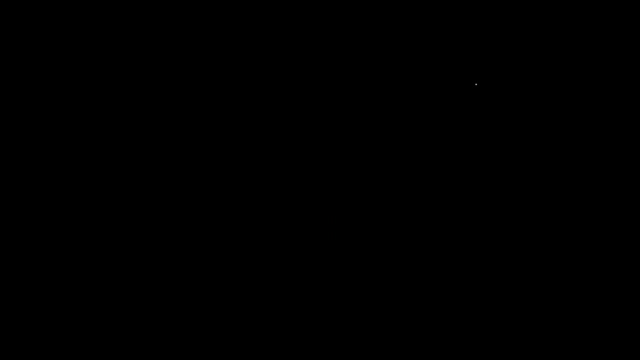 Try this one. Let's say if x is equal to 3 and 2 over 3.. So what you could do is write both equations For this one. let's subtract both sides by 3.. So x minus 3 is equal to. 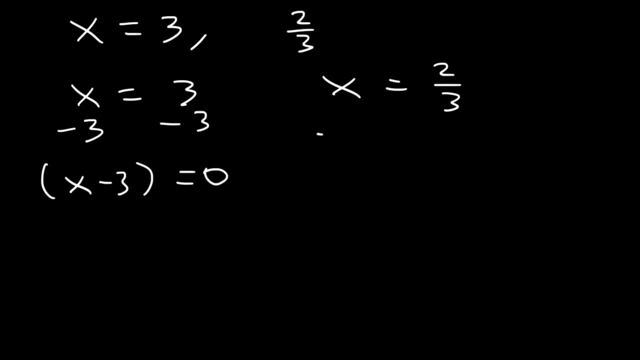 0. That's one of the factors For the other one. if we subtract both sides by 2 thirds, we'll have x minus 2 over 3 is equal to 0.. Now we want to get rid of the fraction, So let's multiply everything by 3.. So 3 times. 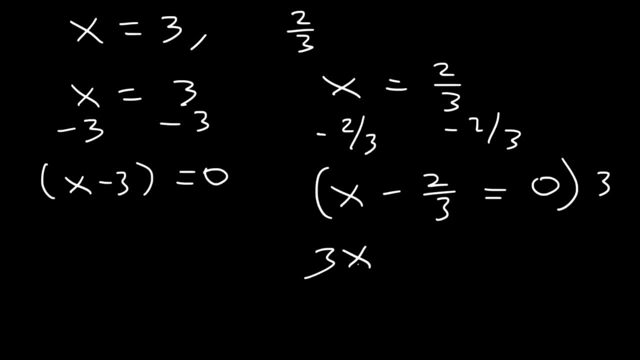 x, that's 3x, And 3 times negative, 2 thirds, that's a negative 2.. The 3's cancel 0 times 3 is 0. So here's the other factor. So in factored form it's x minus 3 times 3x minus. 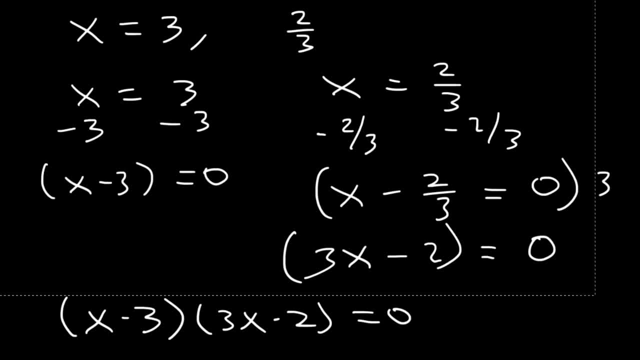 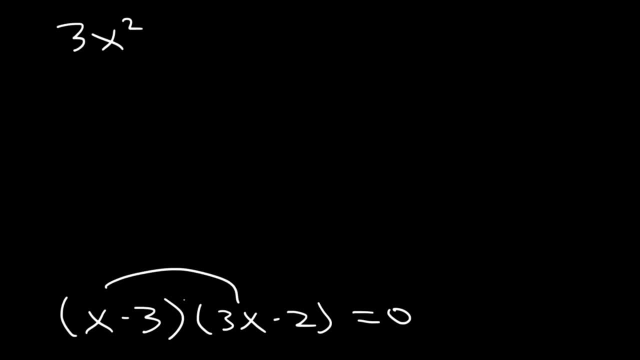 2. So now we can go ahead and FOIL the expression: So x times 3x, that's 3x squared x times negative 2, that's negative 2x. And then we have negative 9x And negative 3 times. 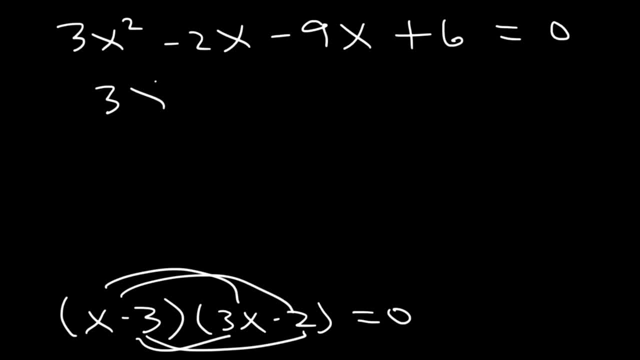 negative 2 is plus 6.. Now, negative 2 minus 9 is negative 11.. And so this is the solution. Now what about this one? Let's say, if you're given just one of the two solutions, How can you write the quadratic equation? Whenever you're dealing with radicals, they always come. 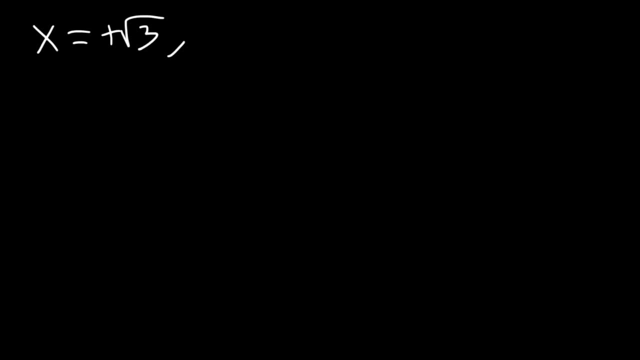 in pairs. So if you have positive root 3, then the other solution must be negative root 3.. So this is going to be x minus root 3 times x plus root 3.. And then you can FOIL: So x times x is x squared, And then x times root 3, that's going to be positive root 3x Negative. 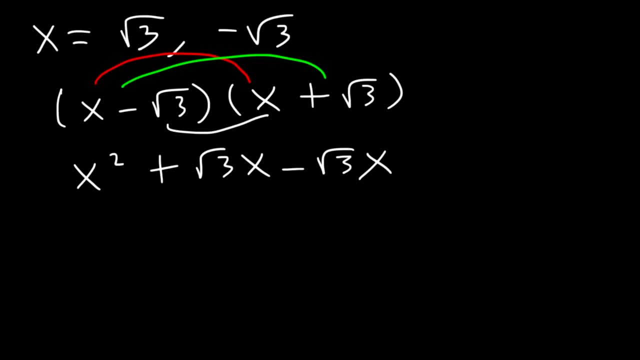 root 3 times x is negative root 3x. Negative root 3 times positive root 3. that's just going to be negative 3.. And the middle terms will cancel. They add up to 0.. So the final answer is: x squared minus 3 is equal. 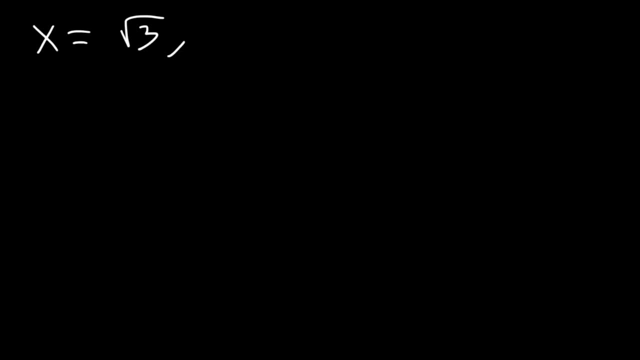 two solutions. how can you write the quadratic equation? whenever you're dealing with radicals, they always come in pairs. so if you have positive root 3, then the other solution must be negative 3. so this is going to be x minus root 2 times x plus root 3. 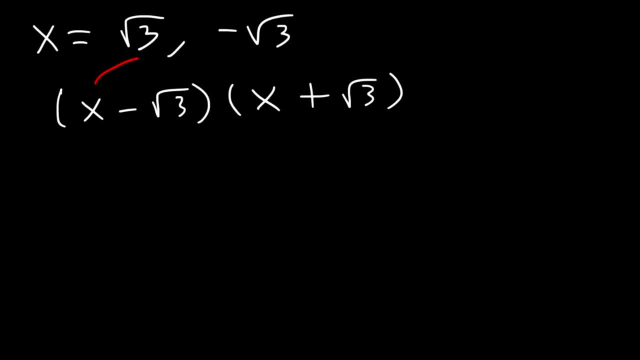 then you can for you. so x times x is x squared, and then x times root 3, that's going to be positive root 3x plus 3x plus root 3x squared. thus X equation, maximum of x squared times x is equal to 0. this is how Xahuas. 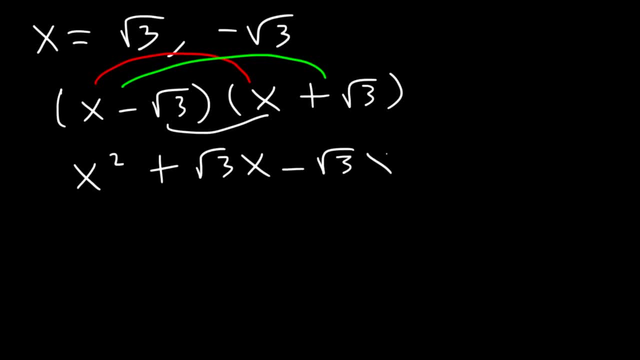 x, negative root 3 times x, negative root 3x, and negative root 3 times positive root 3, that's just going to be negative 3.. And the middle terms will cancel. they add up to 0.. So the final answer is: x squared minus 3 is equal to 0.. 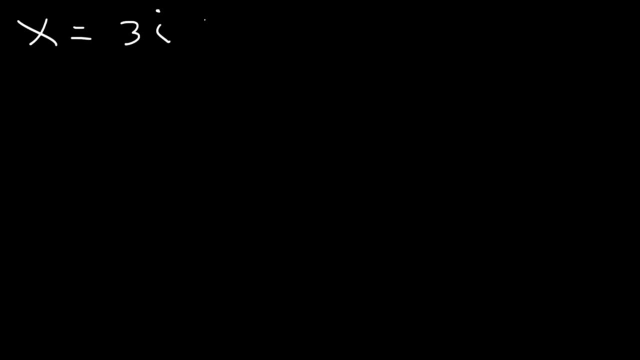 Now the same is true for imaginary numbers. Let's say, if x is equal to 3i, the other solution must be negative 3i. So in factored form it's going to be x minus 3i and x plus 3i. 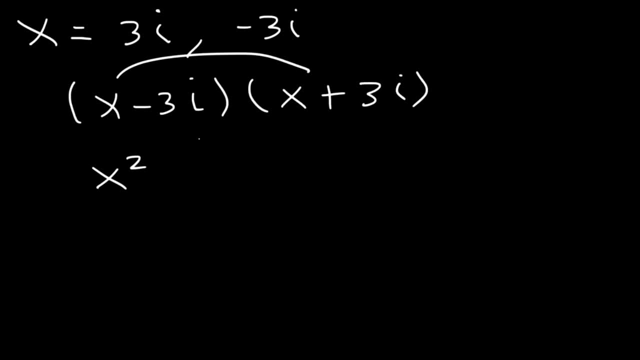 So let's FOIL x times x, that's going to be x squared. and then we're going to have 3ix and then negative 3ix. negative, 3i times positive, 3i. Negative 3 times 3 is negative. 9, i times i is i squared. 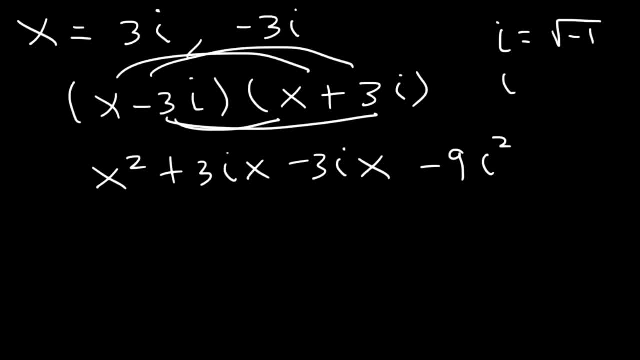 Now keep in mind: i is equal to the square root of negative 1, but i squared is negative 1.. Now the two middle terms. The two middle terms will cancel and let's replace i squared with negative 1.. So negative 9 times negative 1 is positive 9.. 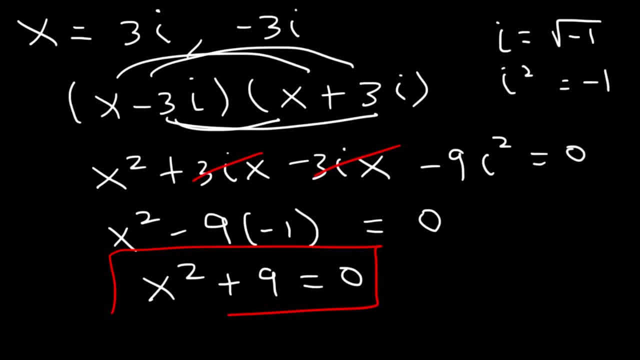 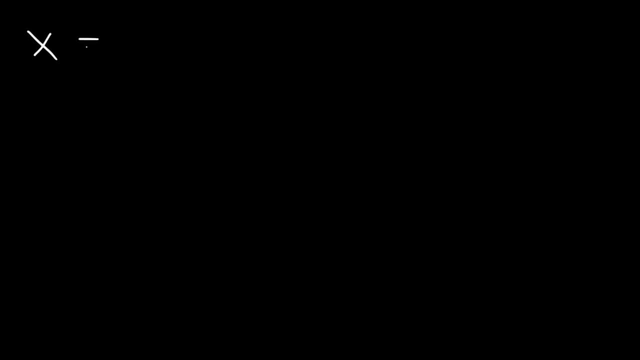 So this is the final answer: x squared plus 9.. Now let's try one more example: 2 plus 3i. What's the other solution? The conjugate of 2 plus 3i is 2 minus 3i. 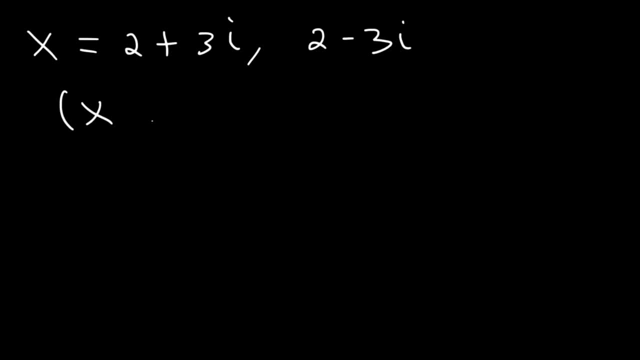 So in factored form it's going to be x. Now notice that the 2 is positive in both cases, so you've got to change the sign. It's going to be x minus 2.. Here we have plus 3i, so you change the sign to minus 3i and the other one is going to. 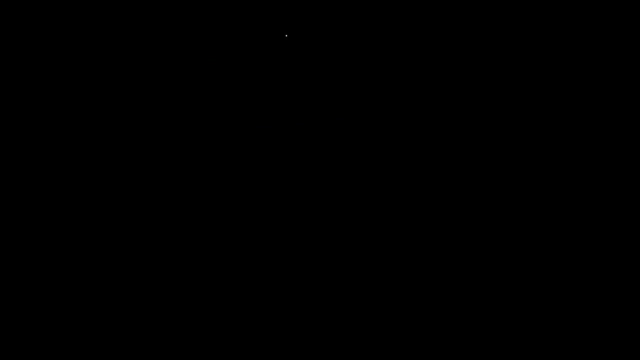 to 0.. Now the same is true for imaginary numbers. Let's say, if x is equal to 3i, the other solution must be negative 3i. So in factored form it's going to be x minus 3i and x plus 3i. 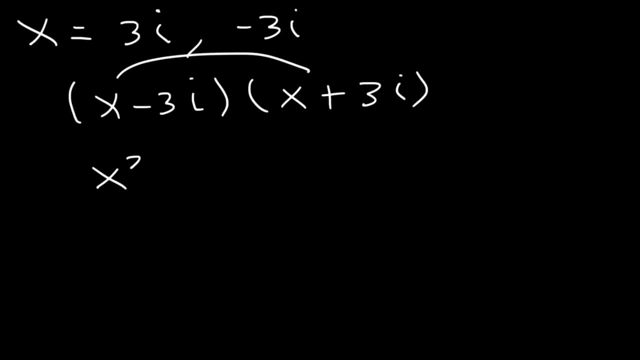 So let's FOIL x times x, that's going to be x squared, And then we're going to have 3ix and then negative 3ix. Negative, 3i times positive. 3i. Negative 3 times 3 is negative, 9.. i times. 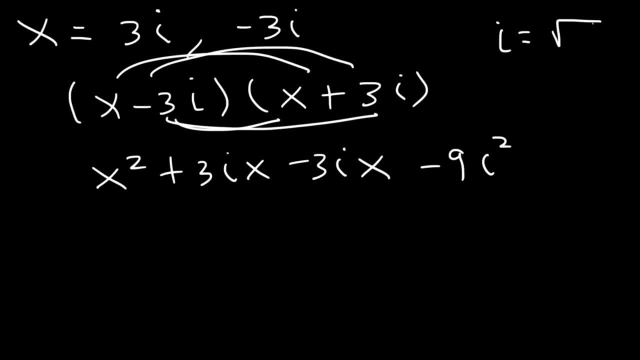 i is i squared. Now, keep in mind i is equal to the square root of negative 1.. But i squared is negative 1.. Now the two middle terms will cancel And let's replace i squared with negative 1.. So negative 9 times negative 1 is positive 9.. So this is the final answer: x squared. 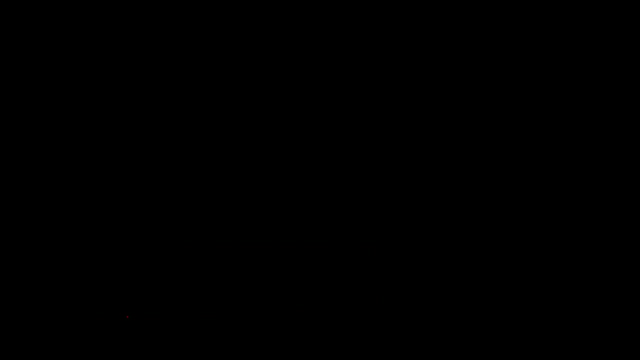 plus 9.. Now let's try one more example: 2 plus 3i. What's the other solution? The conjugate of 2 plus 3i is 2 minus 3i, So in factored form it's going to be x plus 3i. 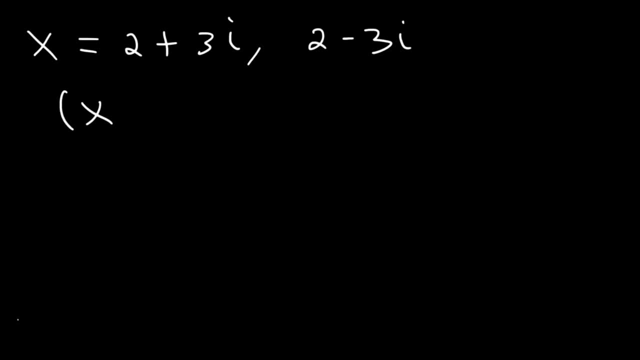 Now notice that the 2 is positive in both cases, So you've got to change the sign. It's going to be x minus 2.. Here we have plus 3i, So you change the sign to minus 3i And the. 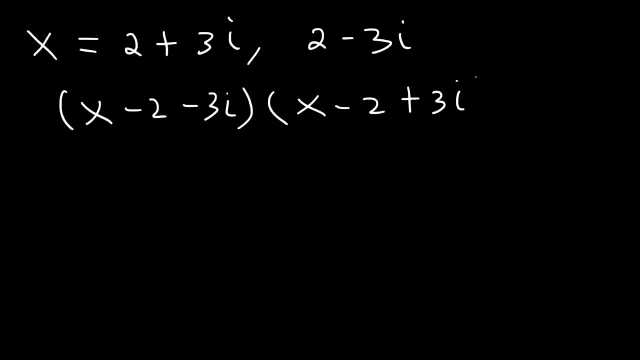 other one is going to be x minus 2 plus 3i. Now we're going to do this two ways, Whenever you FOIL a trinomial with three terms with another trinomial. initially you're going to get nine terms, But there is a shortcut method to doing this factoring problem. I'm 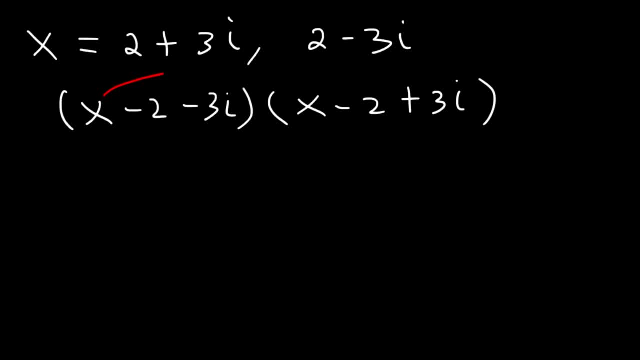 going to do it both ways. So first let's multiply x by x, So that's going to be x squared, And then x times negative 2.. That's negative 2x, And then x times 3i, So that's 3i x. Now let's take negative 2. 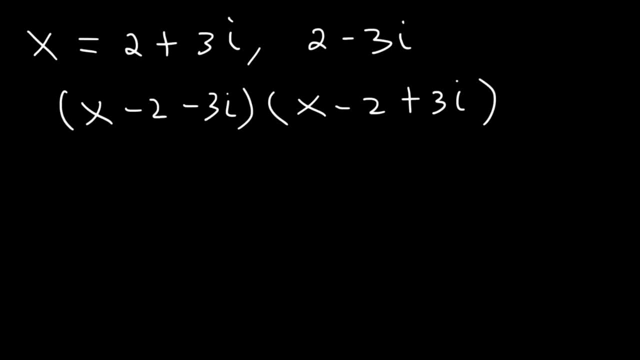 be x minus 2 plus 3i. Now we're going to do this two ways: Whenever you FOIL a trinomial with three terms with another trinomial. initially, you're going to get nine terms, But there is a way to do this. 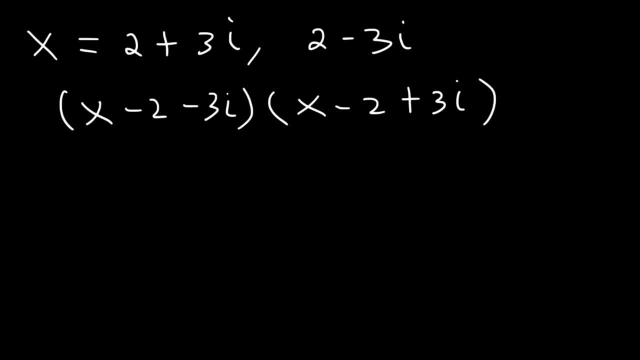 Here's a shortcut method to doing this factoring problem, but I'm going to do it both ways. So first let's multiply x by x, So that's going to be x squared, And then x times negative 2, that's negative 2x, and then x times 3i. 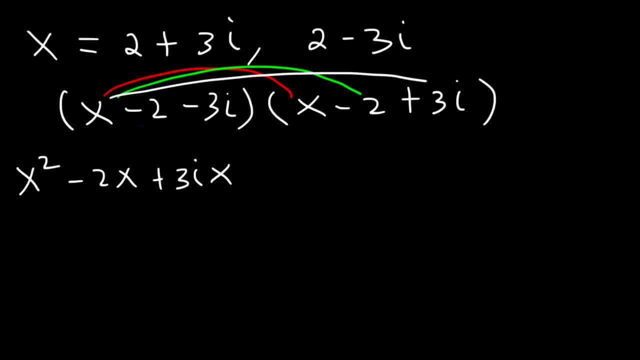 So that's 3i- x. Now let's take negative 2 and multiply by x, So that's negative 2x, And then negative 2 times negative, 2 is positive 4.. Negative 2 times 3i is negative 6i. 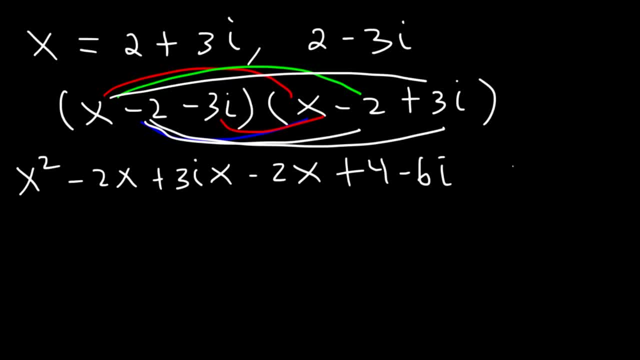 Now let's take negative 3i and multiply by x, That's negative 3i, x, And then negative 3i times negative 2,, that's positive 6i. And then the last one, negative 3i times negative 3i, that's negative 9i squared. 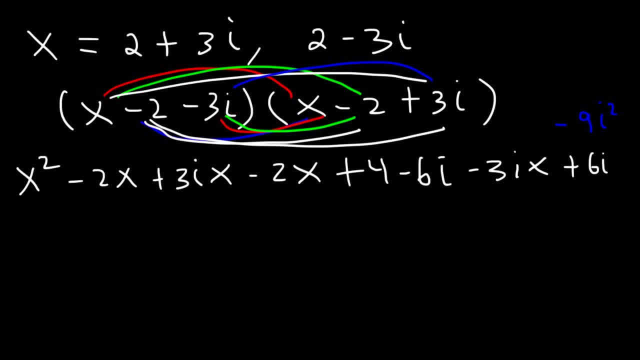 So notice that initially we have nine terms. Now let's cancel 3i x and negative. 3i x will cancel And negative 6i plus 6i will cancel. Now we can combine negative 2x and negative 2x. 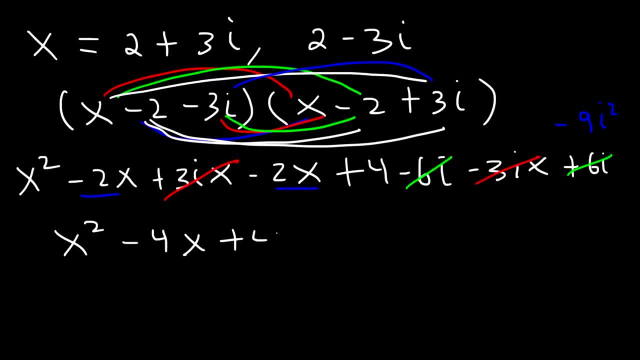 So it's x squared minus 4x plus 4.. And we know that i squared is negative 1, so negative 9i squared is negative 9 times negative 1, which is plus 9.. So it's going to be x squared minus x squared, plus x squared minus x squared, so that's. 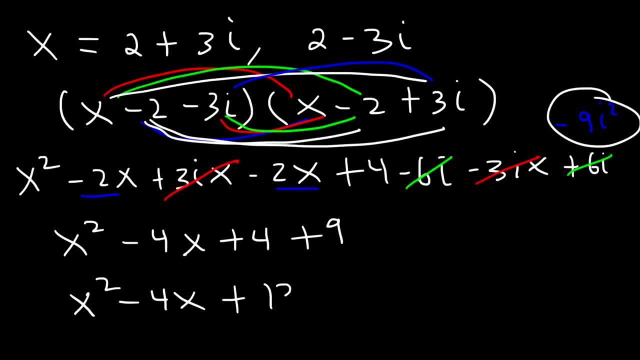 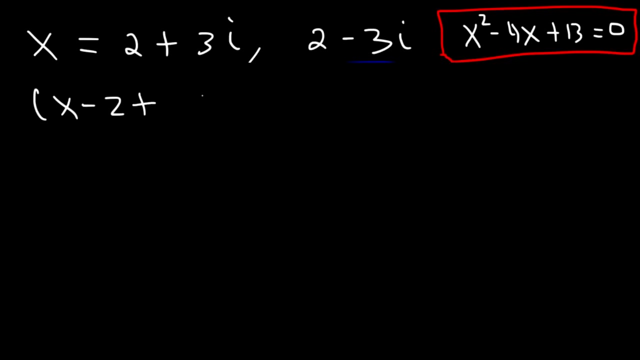 minus 4x, and 4 plus 9 is 13. so that's the answer. x squared minus 4x plus 13 is equal to 0. now let's get the same answer using another technique, which will save you some time. so, in factored form, this is the answer: x minus 2 plus 3i and x. 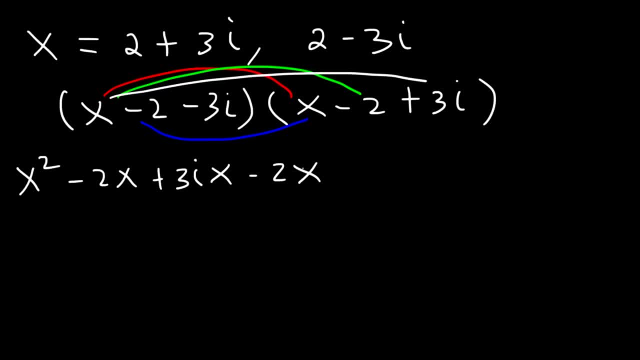 and multiply by x, So that's negative 2x, And then negative 2 times negative, 2 is positive 4.. Negative 2 times 3i is negative 6i. Now let's take negative 3i and multiply by x, That's negative 3i, x And then negative. 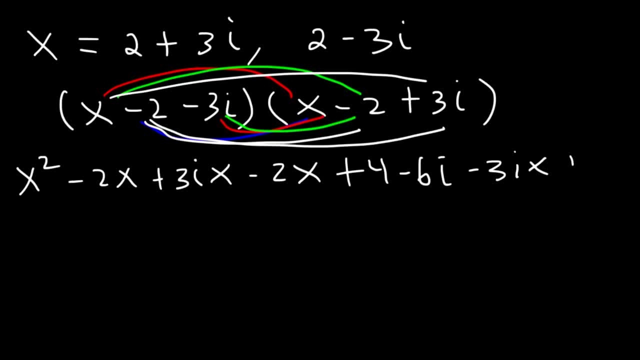 3i times negative 2.. That's positive 6i. And then the last one, negative 3i times negative 3i. That's negative 9i squared. So notice that initially we have nine terms. Now let's: 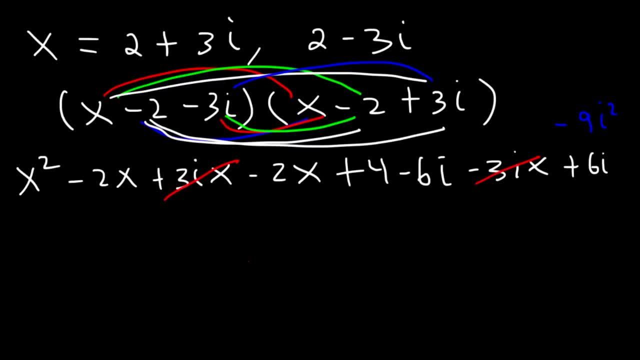 cancel 3i- x and negative 3i- x will cancel, and negative 6i plus 6i will cancel. now we can combine negative 2x and negative 2x, so it's x squared minus 4x plus 4, and we know that i squared is negative 1, so negative 9 i. 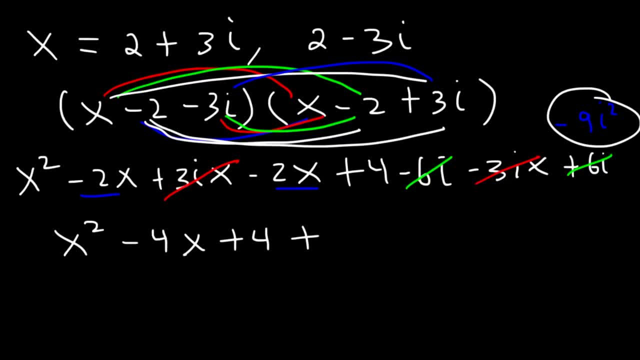 squared is negative, 9 times negative 1, which is plus 9. so it's going to be x squared minus 4x, and 4 plus 9 is 13. so that's the answer. x squared minus 4x plus 13 is equal to 0. 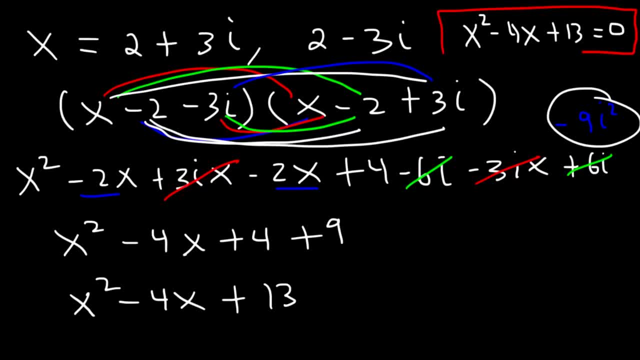 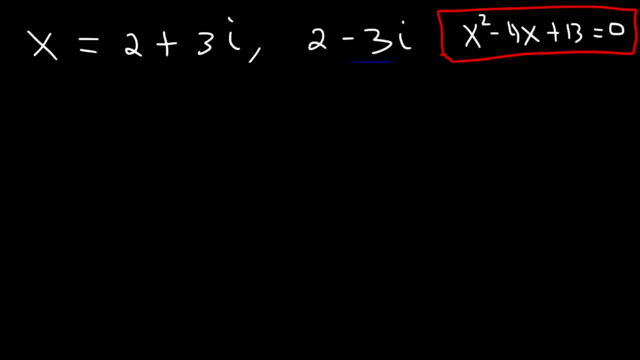 now let's get the same answer using another technique, which will save you some time. so, in factored form, this is the answer: x minus 2 plus 3i and x minus 2 minus 3i. it turns out that and that expression is equivalent to x minus 2, squared plus 3i, times negative 3i. Now, if we FOIL x minus 2, 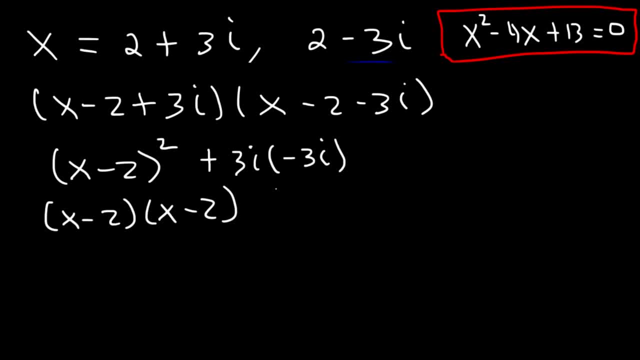 times x minus 2 and 3i times negative 3i. we know it's negative. 9i squared x minus 2 times x minus 2 is x squared minus 4x plus 4.. And negative 9i squared is positive 9.. And 4 plus 9 is 13.. 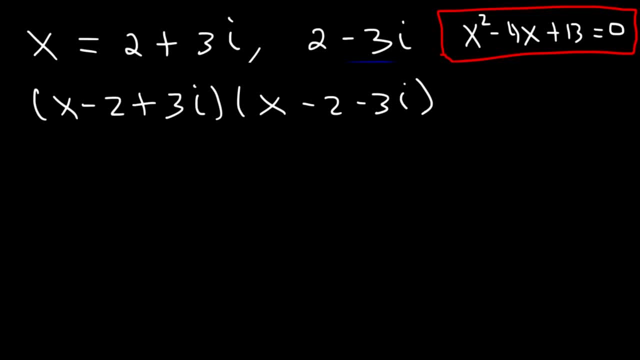 minus 2 minus 3i, it turns out that and that expression is equivalent to x minus 2 squared plus 3i times negative 3i. now if we FOIA x minus 2 times x minus 2 and 3i times negative 3i, we know it's a negative 9i squared x minus 2 times x. 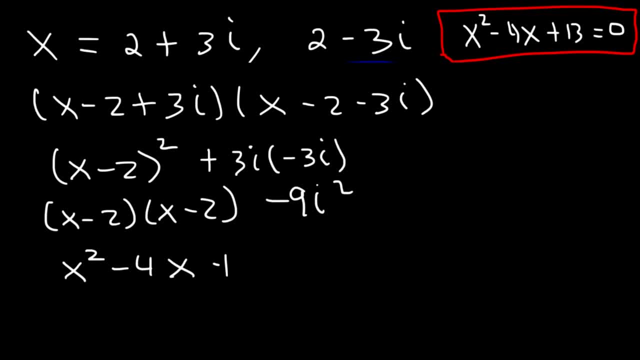 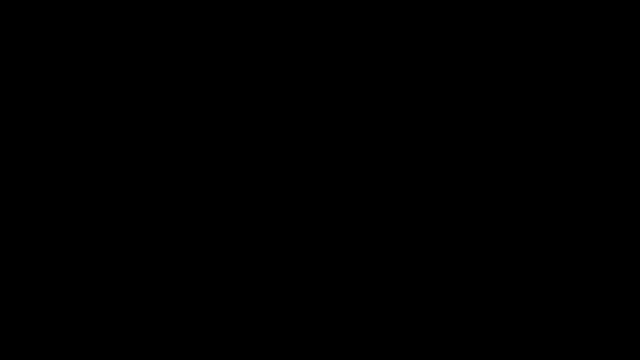 minus 2 is x, squared minus 4x plus 4 and negative 9i squared is positive 9 and 4 plus 9 is 13. so, as you can see, you can get the same answer but much faster using that technique. now, sometimes you might be given three points. let's say if: 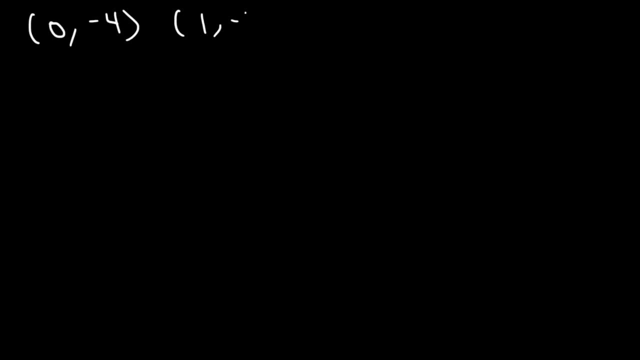 you have the point 0 negative 4, 1 negative 1 and 2 negative 10. write a quadratic equation in standard form, given these three points. so the standard form of a quadratic equation is: ax squared plus B, X plus C is equal to 0. so 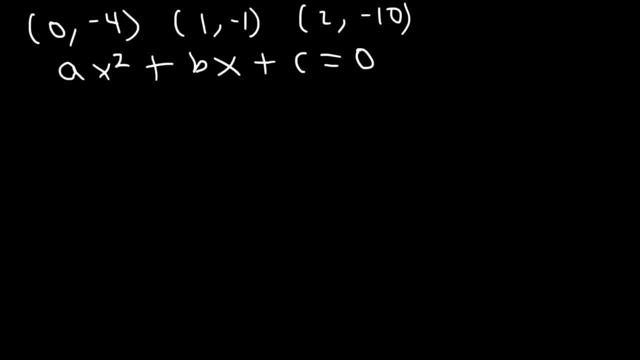 we got to find the values of a, B and C. actually, rather than equaling 0, this is all equal to Y. so let's start with the first point: 0 negative 4, X is 0 and Y is negative 4. so let's replace Y with negative 4 and X with 0. 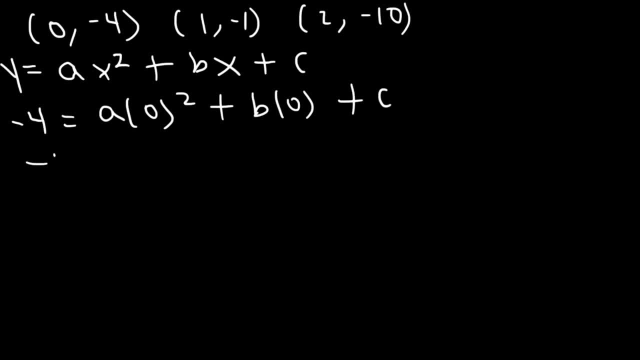 if we do that, we can see that negative 4 is equal to C. so that's the first answer. now let's find a and B. now let's use the second point. Y is negative 1 when X is 1, so therefore negative 1 is equal to 0 and X is equal to 0. so that's the first answer. now let's 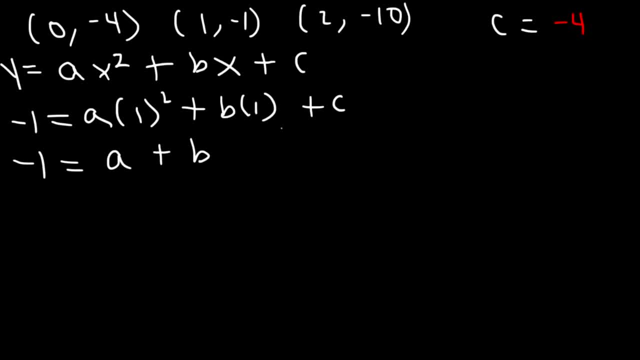 use negative 1. this one is the second and third part, so let's use the second and so let's do this. so negative 1 is equal to a plus B, and we know C is negative 4. so if we add 4 to both sides, then we can see that a plus B is equal. 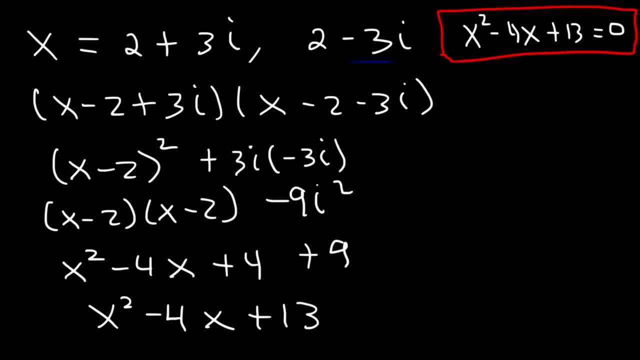 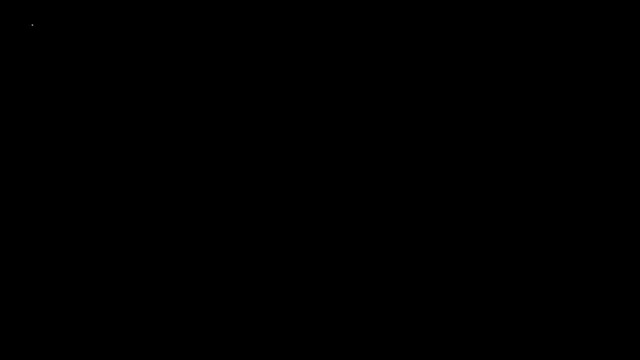 So, as you can see, you can get the same answer but much faster using that technique. Now, sometimes you might be given three points, Let's say, if you have the point 0, negative, 4, 1, negative 1, and 2, negative 10.. Write a quadratic equation in standard form. 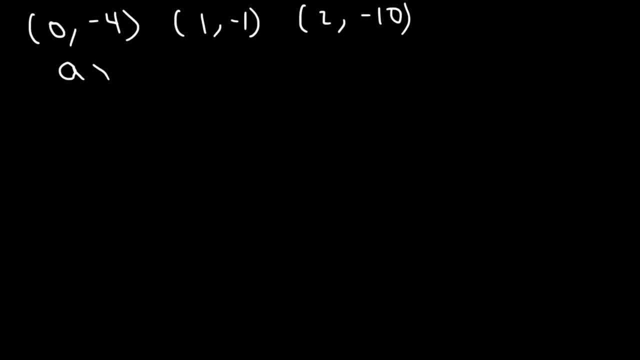 given these three points. So the standard form of a quadratic equation is ax squared plus bx plus 3i squared, And if you have a quadratic equation, you can write a quadratic equation in standard form, given these three points. So we have to find the values of a, b and c, Actually, rather than equaling 0,. this is all. 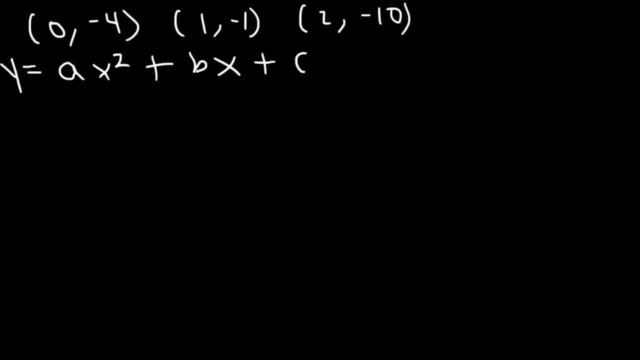 equal to y. So let's start with the first point: 0, negative 4.. x is 0 and y is negative 4.. So let's replace y with negative 4 and x with 0. If we do that, we can see that negative 4 is equal to c. 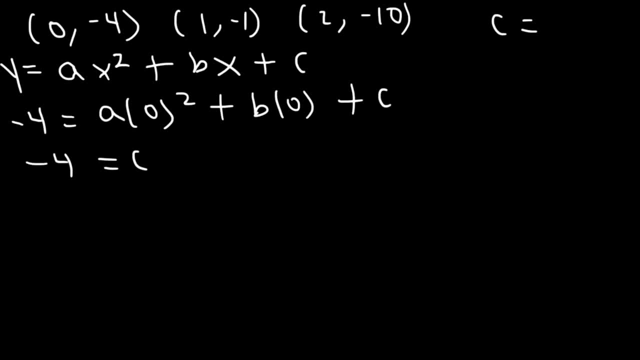 So let's replace y with negative 4 and x with 0.. If we do that, we can see that negative 4 is equal to c. So that's the first answer. Now let's find a and b. Now let's use the second point. y is negative 1 when x is 1.. 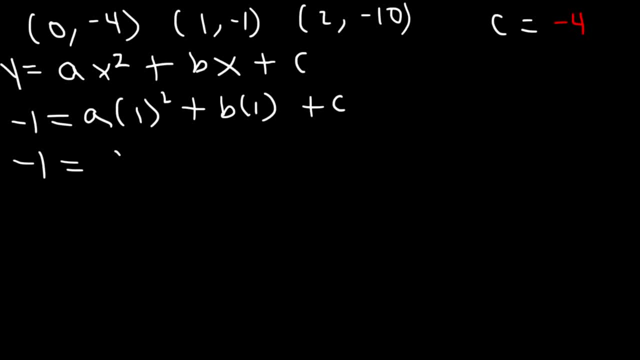 So therefore negative 1 is equal to a plus b, and we know c is negative 4.. So if we add 4 to both sides, then we could see that a plus b is equal to negative 1 plus 4, which is 3.. 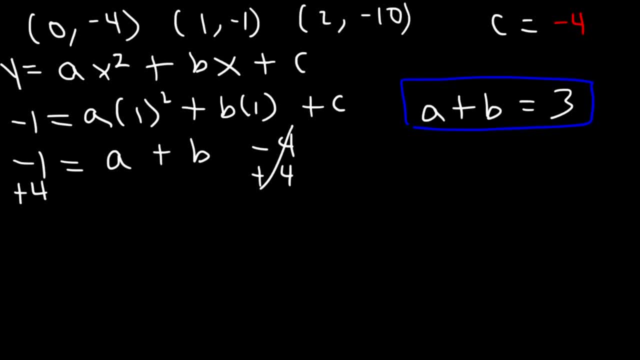 So let's save this equation. We're gonna use it later. Now let's use the second equation—or rather the third point—to get another equation in terms of a and b. So x is to y is negative 10.. So negative 10 is equal to a times 2 squared plus b squared. 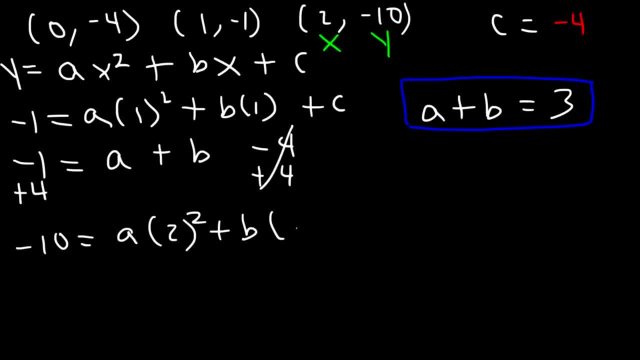 x is to y is negative 10.. So negative 10 is equal to a times 2 squared plus b squared. So negative 10 is equal to a times 2 squared plus b squared times 2 plus C. Now 2 squared is 4, and C is negative 4.. So let's add 4 to both sides. 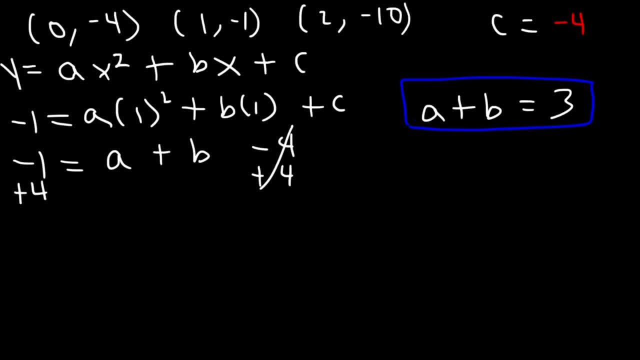 to negative, 1 plus 4, which is street. so let's say this equation, we're going to use it later. now let's use the second equation, or rather I mean the third point, to get another equation in terms of a and B. so is equal to a times 2 squared plus b, times 2 plus c. Now 2 squared is 4 and c is negative. 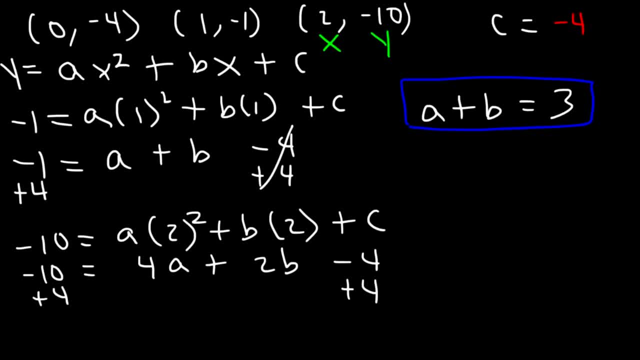 4.. So let's add 4 to both sides. Negative 10 plus 4 is negative 6.. So negative 6 equals 4a plus 2b. So I'm going to write it here: 4a plus 2b is equal to negative 6.. Now that 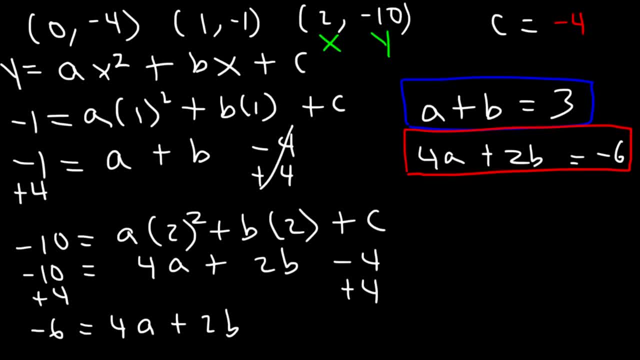 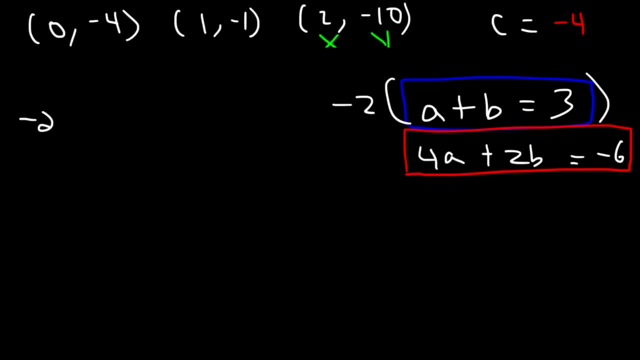 we have two equations and two variables. we can use elimination to solve for a and b. So let's multiply the first equation by negative 2 to cancel the b. So negative 2a minus 2b is equal to negative 6.. And 4a plus 2b is also equal to negative 6.. So if we add these, 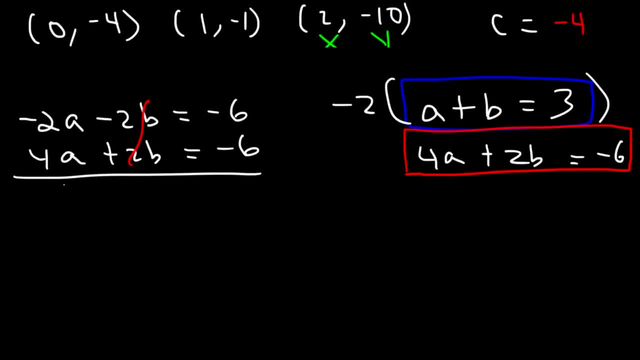 two equations, 2b and 2b will cancel Negative. 2a plus 4a is 2a, Negative 6 plus 6 is negative 12.. Next, let's divide by 2.. So a is negative 12 divided by 2, which is negative 6.. 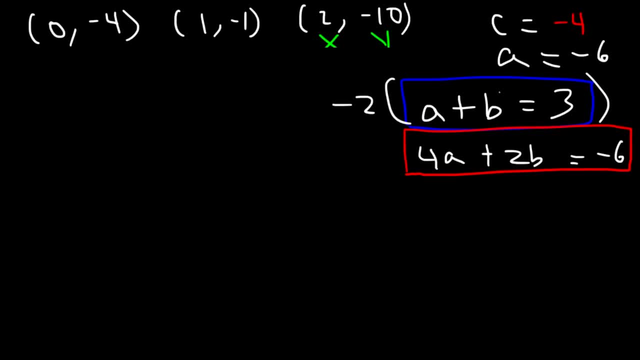 Now let's find the value of b And let's use the first equation in its unmodified form. So a plus b is equal to 3. And a is negative 6. So if we add 6 to both sides, we can see that b is 3 plus 6, which is 9.. 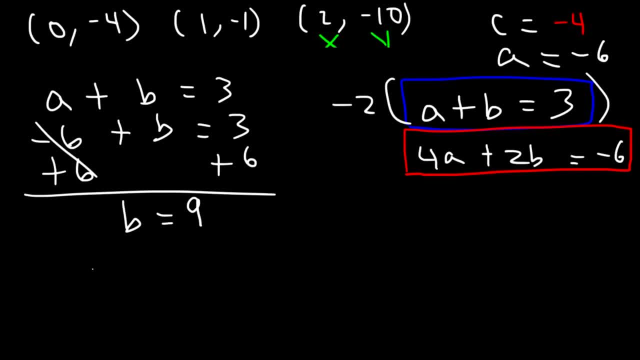 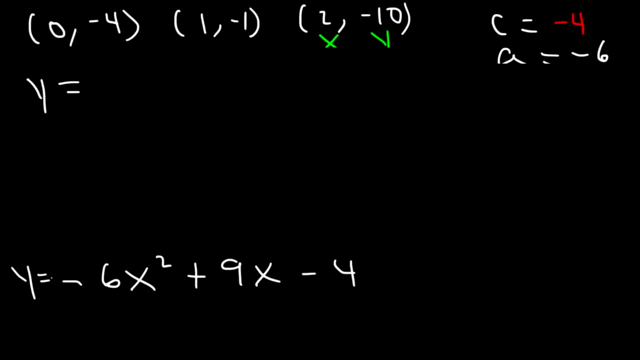 So, therefore, the equation is going to be negative: 6x squared plus 9x minus 4.. Now what we need to do is make sure the work is correct, So let's check it. So let's start by plugging in the first point: 0, negative 4.. 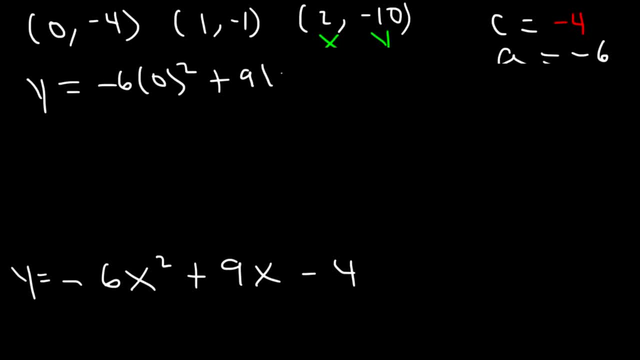 Negative 6 times 0. squared plus 9 times 0 minus 4 will be negative 4.. So we do indeed get the y value here. Now let's try the point 1, negative 1.. When we plug in 1, we should get a y value of negative 1.. 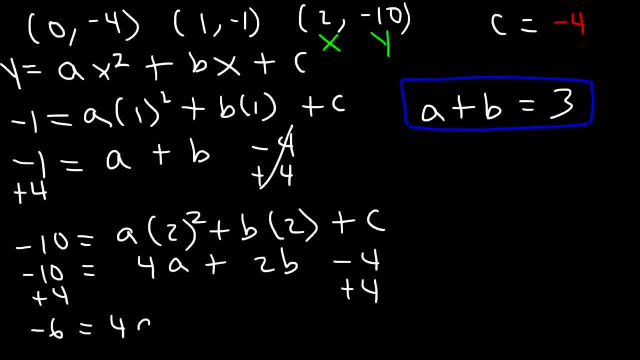 Negative 10 plus 4 is negative 6.. So negative 6 equals 4A plus 2B. So I'm going to write it here: 4A plus 2B is equal to negative 6.. Now that we have two equations and two variables, 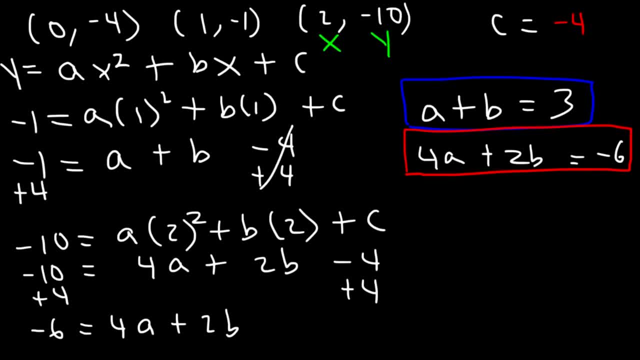 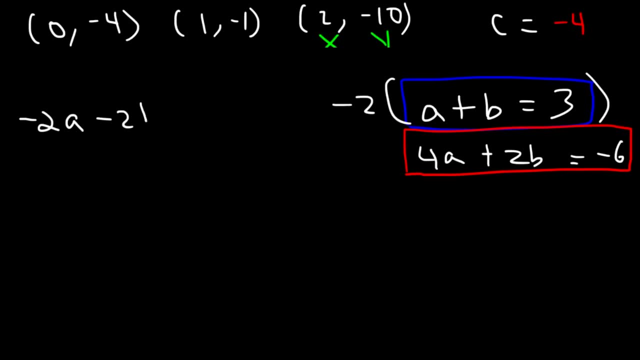 we can use elimination to solve for A and B. So let's multiply the first equation by negative 2 to cancel B. So negative 2A minus 2B is equal to negative 6.. And 4A plus 2B is also equal to negative 6.. So if we add these two equations, 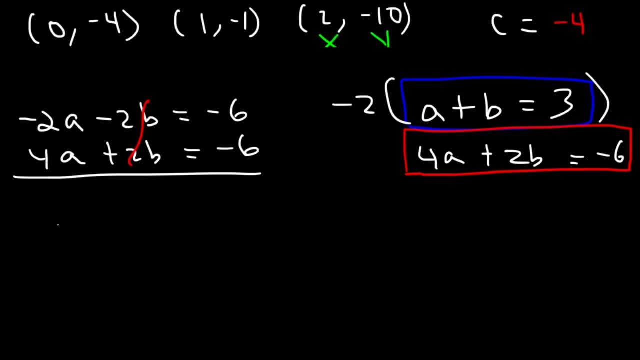 negative 2B and 2B will cancel Negative. 2A plus 4A is 2A. Negative 6 plus 6 is negative 12.. Next let's divide by 2.. So A is negative 12 divided by 2, which is negative 6.. 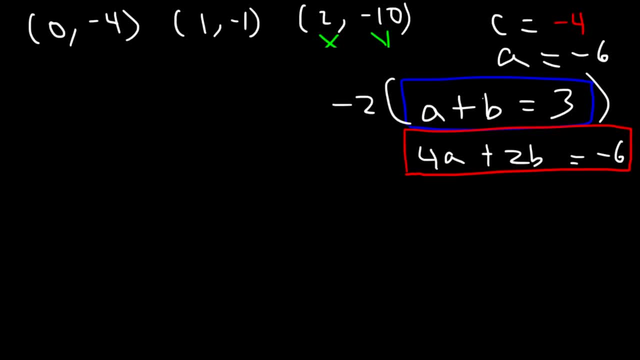 Now let's find the value of B And let's use the first equation in its unmodified form. So A plus B is equal to 3. And A is negative 6. So if we add 6 to both sides, we get negative 6.. 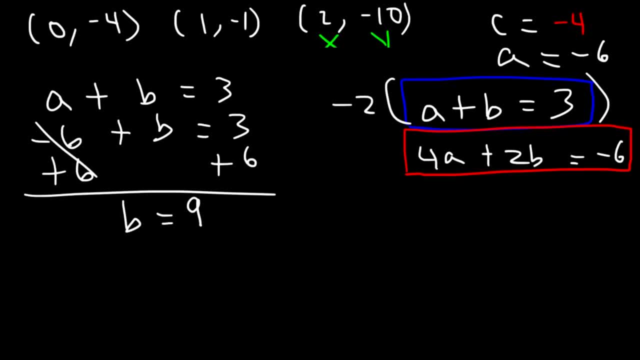 We can see that B is 3 plus 6, which is 9.. So, therefore, the equation is going to be negative: 6x squared plus 9x minus 4.. Now what we need to do is make sure the work is correct. So let's check it. 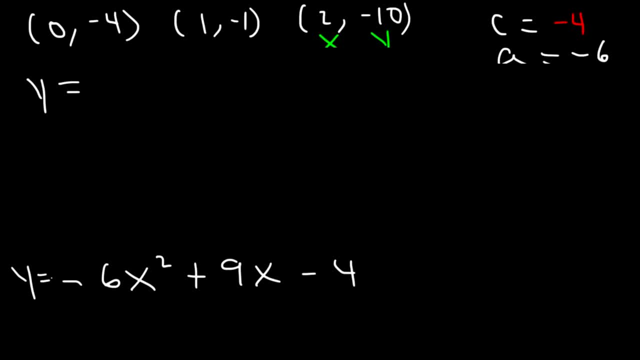 So let's start by plugging in the first point: 0, negative 4.. Negative 6 times 0 squared plus 9 times 0 minus 4 will be negative 4.. So we do indeed get the y-value here. Now let's try the point 1, negative 1.. 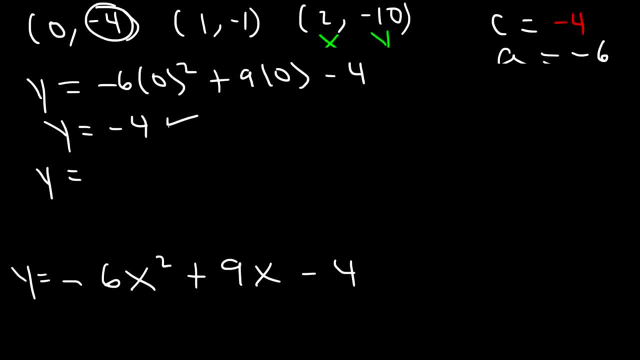 When we plug in 1, we should get a y-value of negative 1.. 1 squared is 1 times negative 6.. That's negative 6.. 9 times 1 is 9.. Negative 6 plus 9 is 3, and 3 minus 4 is negative 1.. So that works.